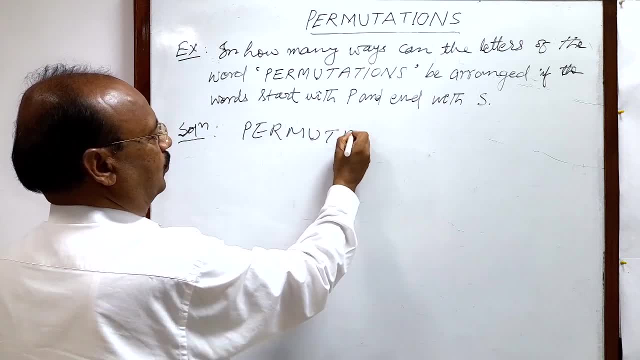 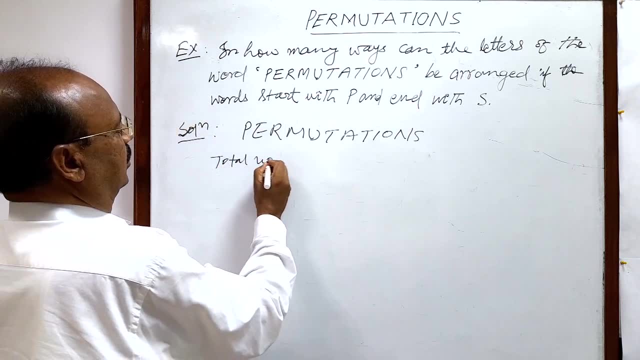 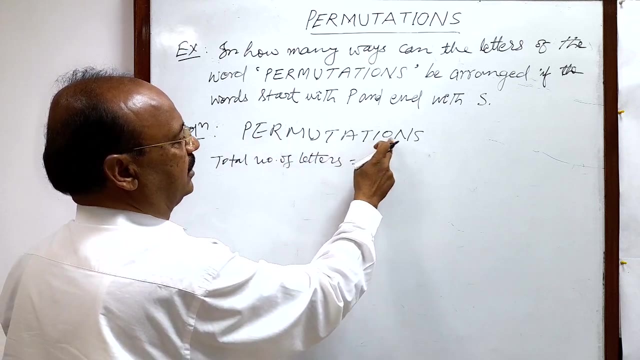 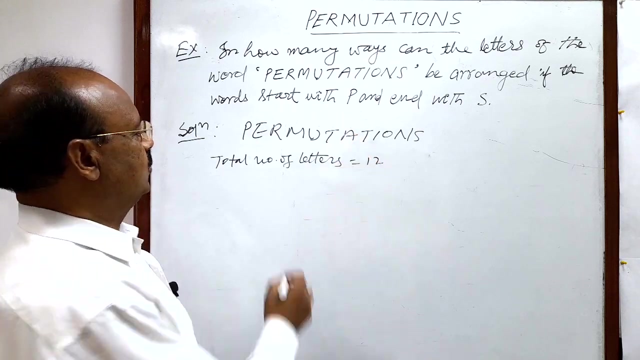 And here total number of letters. total number of letters, how many? 1, 2,, 3,, 4,, 5,, 6,, 7,, 8,, 9,, 10,, 11,, 12.. Okay, and there is a repetition of 2, sorry, repetition of T, twice So number of T's. 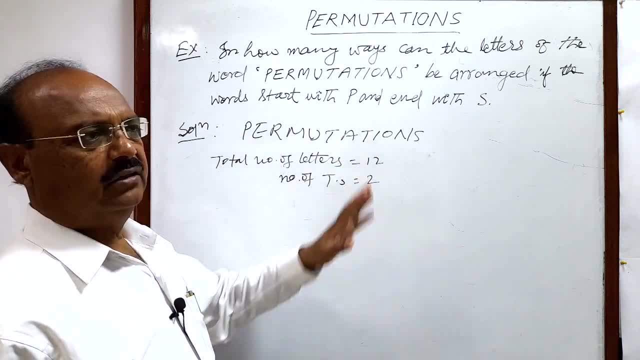 is 2.. And rest of the letter is 2.. So number of T's is 2.. So number of T's is 2.. So number of letters are distinct. Rest of the letters are different. Okay, So here we are going to use a. 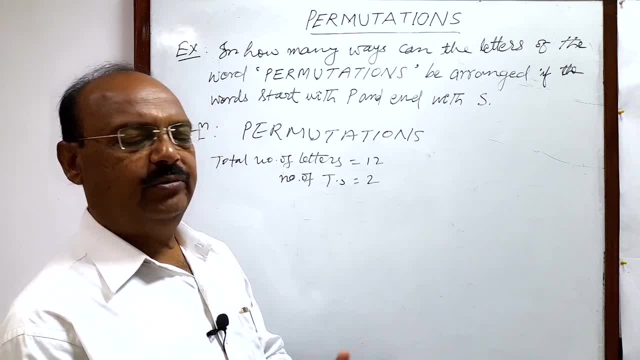 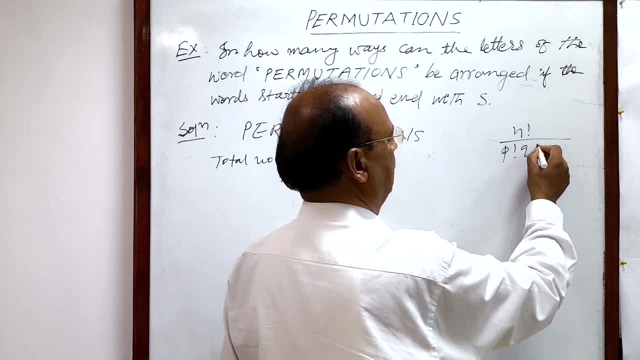 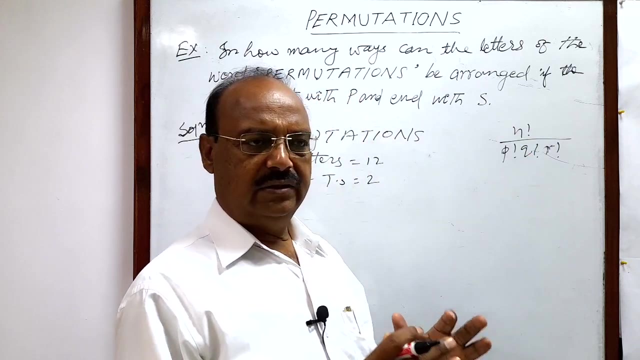 formula that we have studied, we have discussed several times in solving other problem also, which is like this: N factorial by P factorial, Q factorial, R factorial, where N is the total number of objects given And P is the number of objects which are alike of one kind. This is 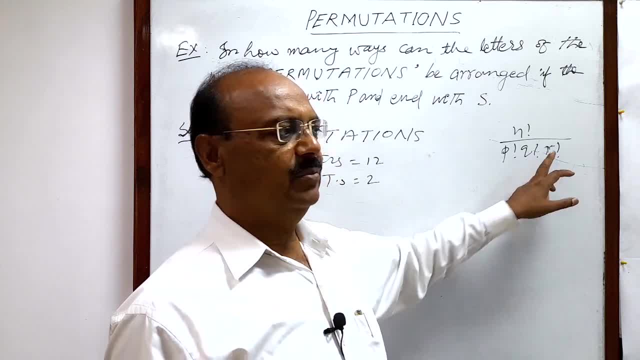 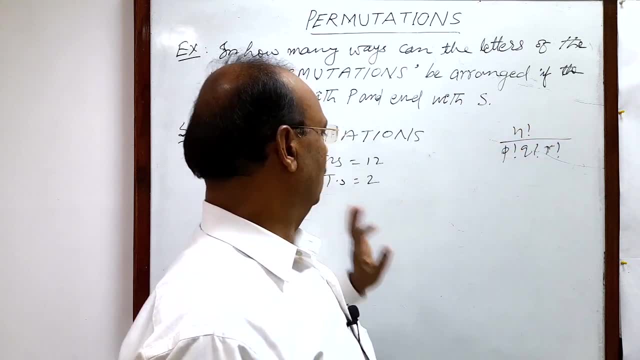 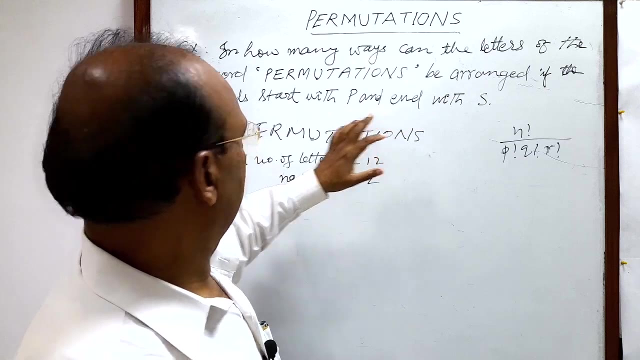 number of objects which are alike of one kind, And P is the number of objects which are alike of objects alike of second kind. This is, R is number of objects alike, isn't it? So we can use this formula here. Correct, Here, total number of letters is 12.. But the condition is here that words should: 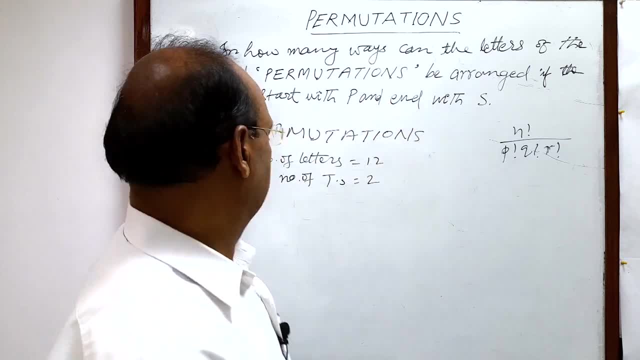 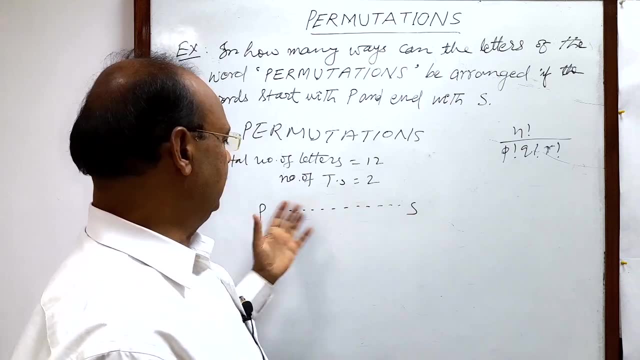 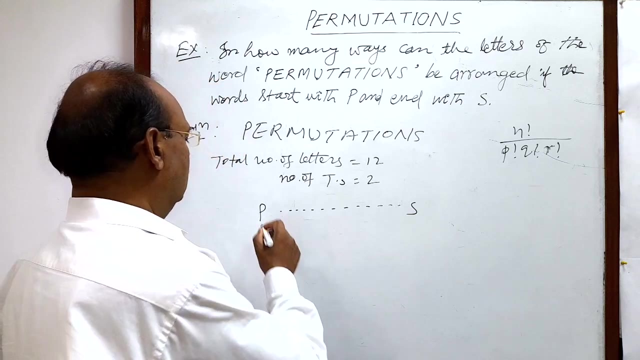 start with P and end with S, So between P and S. all the letters are here lying between P and S, Starting with P and ending with S. So total number of letters will be now how much? Now we will not consider these two letters, because places of these two letters are fixed, Okay So? 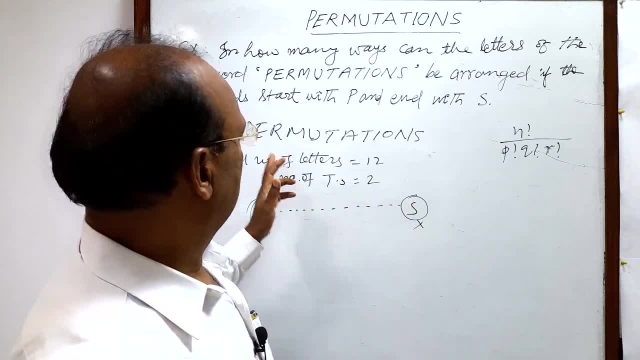 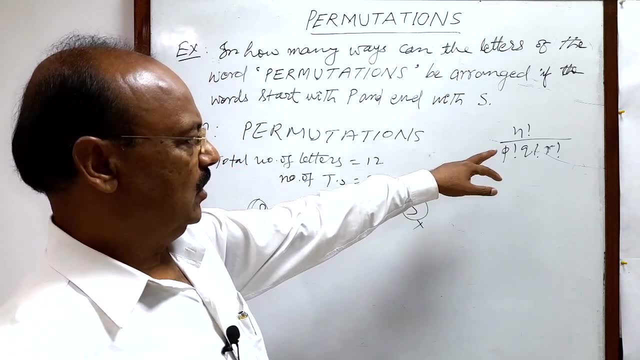 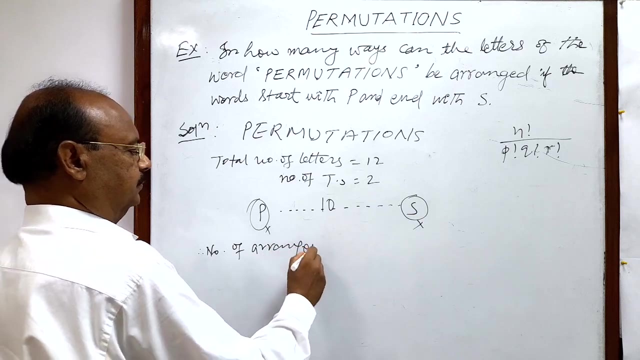 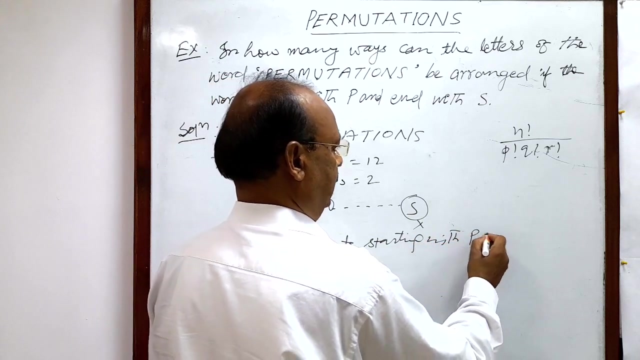 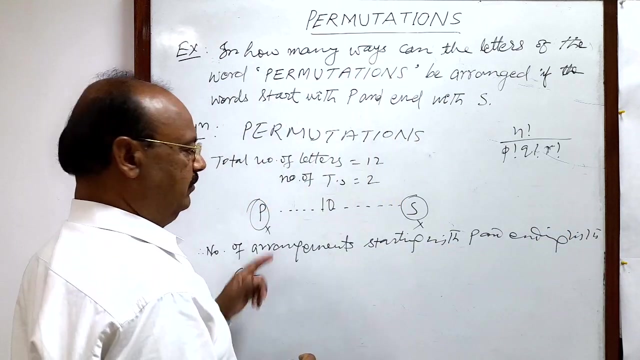 other than these two letters. remaining letters is how many Out of 12,? two letters are fixed, So remaining letters are 10.. Okay, So by this formula, therefore, number of arrangements starting with P and ending with S will be how much N factorial means 10 factorial divided by?